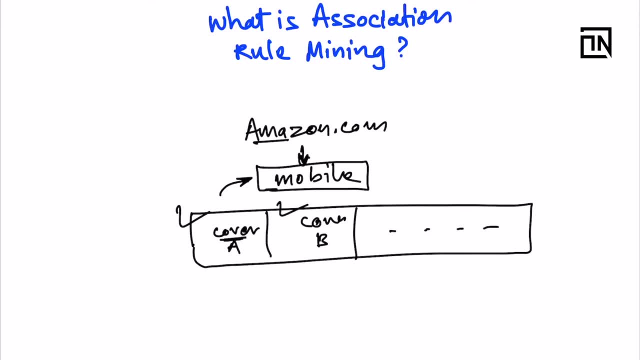 covers. these mobile covers are the one people purchased with this particular mobile phone. Let's say you're taking an iPhone, So for, with iPhone, which particular brand of iPhone mobile cover is very popular amongst everyone? that will be recommended. So how this data is generated. Now 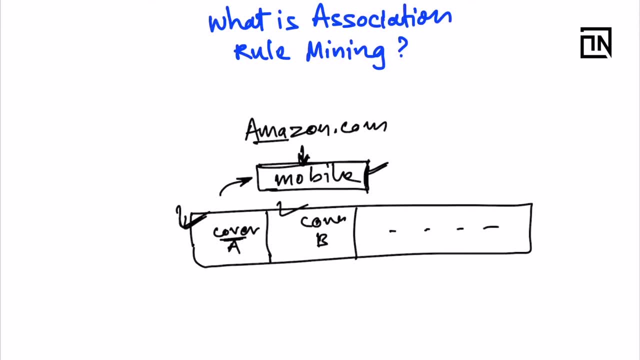 if you think about it, this is just one such example, Like it could be mobile phone, it could be a speaker system, it could be a particular Apple or any any XYZ product. you get these recommendations. So these recommendations are generated partly by association, rule mining and 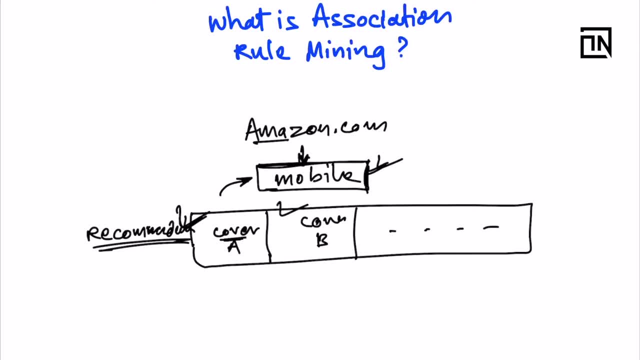 partly by collaboration. So these recommendations are generated partly by association rule mining, separately filtering. But since we are talking about association rule mining, so I'll focus onto the concepts over here Now. so this is one product. Now imagine the number of products at. 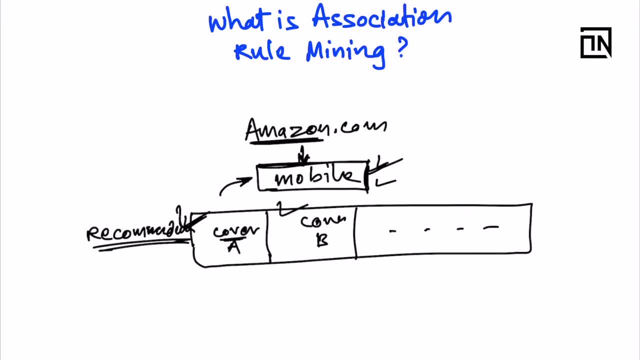 amazoncom. So there are so many millions and millions of different products. So for each one of them, even a team of 1000 or 10,000 or 2000,. 20,000 people will take a lot of time to sort all. 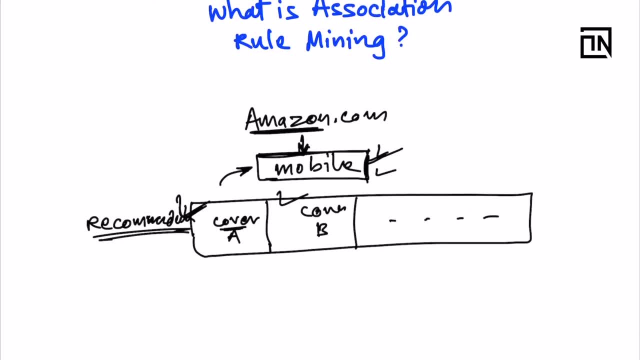 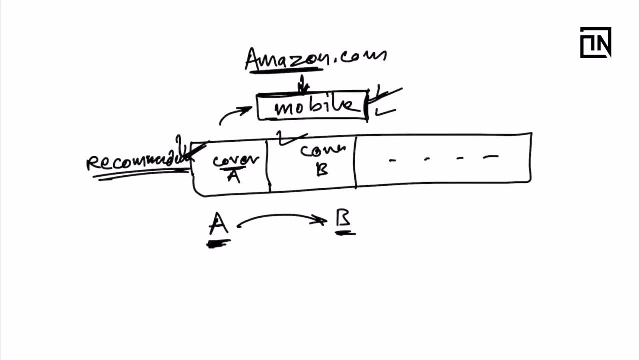 these products and create these kinds of recommendations, Like when the person purchases product A, then recommend the person purchase product B- a very common example when you go to a superstore. So a very, very famous combination is: people who purchase milk will also purchase bread with it- Very common. 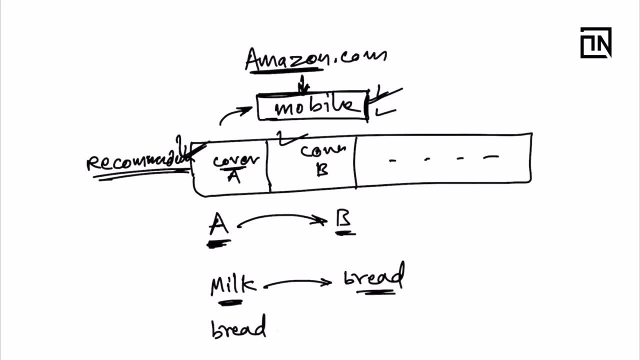 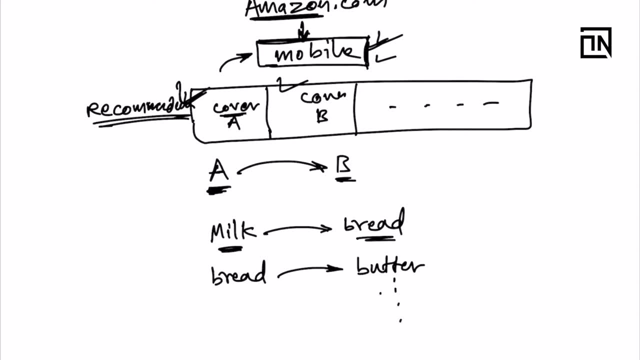 by very common purchase, or people who purchase bread will likely purchase butter with it Or any XYZ product which you like a lot. So these are like. these are behavioral insights which we are trying to derive, The shopping behavior insights which we are trying to derive from the transactions data, Like customer. 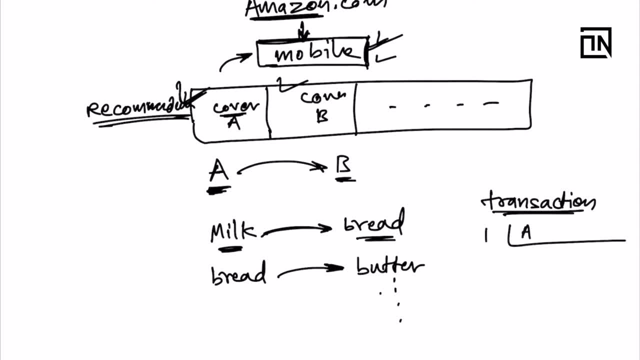 number one purchased the item number A, item number B, item number C, item number D. customer number two purchased item number C, item number D, item number E, so on and so forth. So I have all the transactional transaction data for all the customers in my superstore. So from that I can. 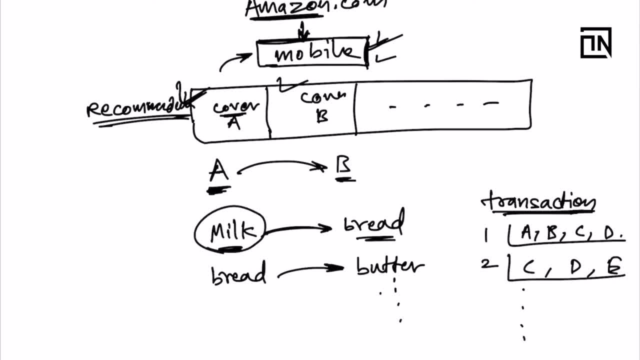 analyze that. okay, people who are who are purchasing milk, they are also going for bread many times. people who are purchasing milk, they are also going for bread many times. people who are purchasing bread, they are going for butter many times. So so this is kind of a rule. This is an 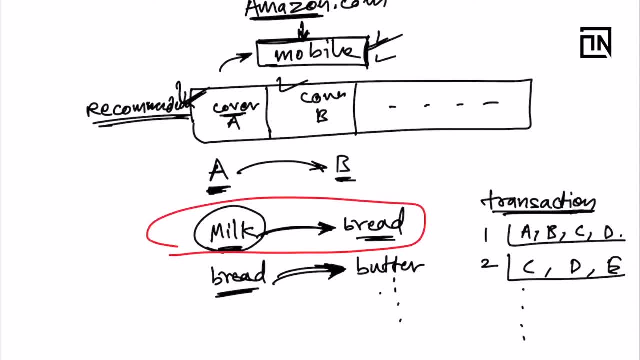 example of a rule that a person who is buying this product A is likely to buy the product B also. there is a probability that if you recommend them, they will buy B also. if you recommend them at the right time, like twice checking out for a particular mobile phone, if you show a cover which 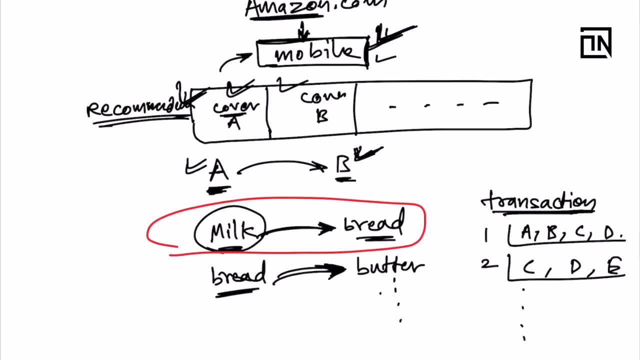 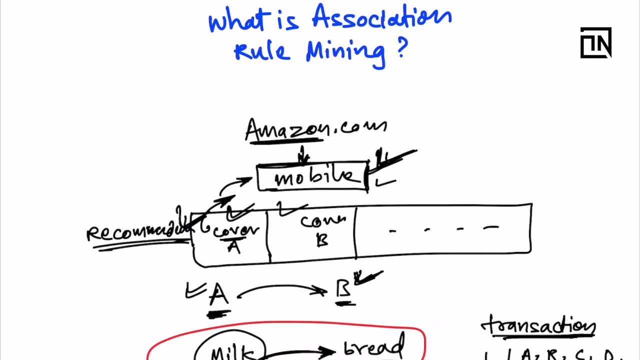 is really great. people really loved it, So there is a high likelihood that the person will also add this and, effectively, your sales will increase. So, ultimately, association rule. mining or, as such, any algorithm or any technique is aimed at increasing the sales, So association rule. 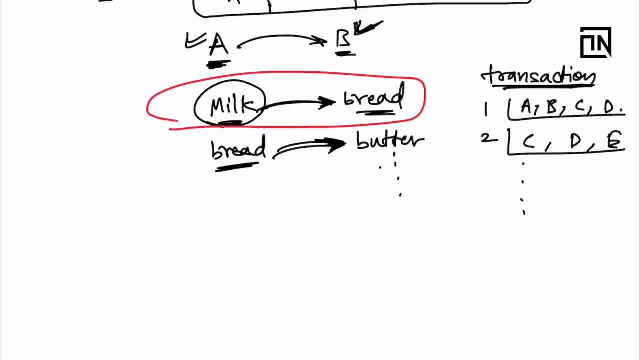 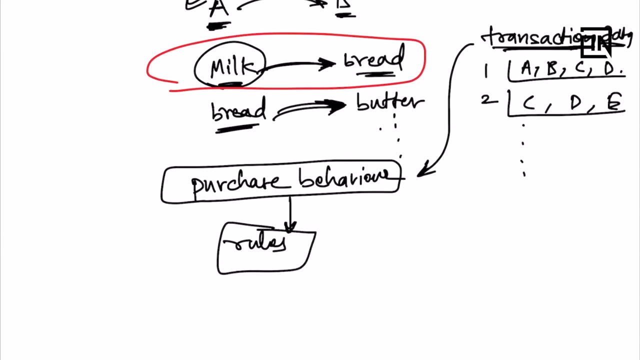 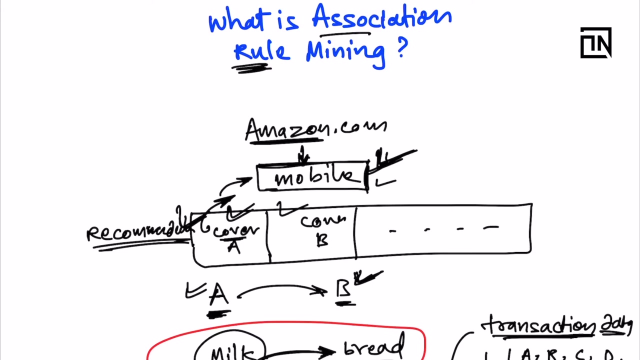 mining helps us find the consumer purchase behavior. based out of what? based out of transaction data. So, using transaction data, we try to analyze the purchase behavior And using purchase behavior analysis, we create certain rules, and these rules are nothing but your association rules, okay, so association rule mining is the procedure or way to find out or to mine the kind of rules. 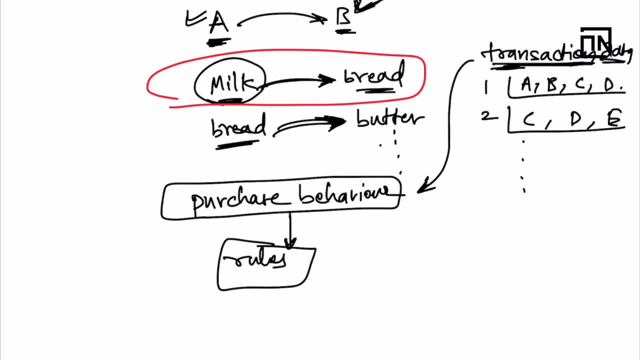 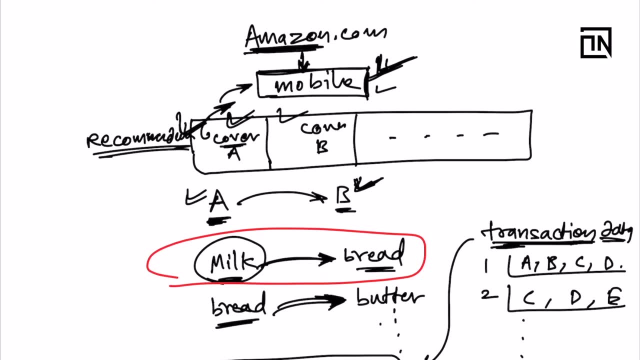 which are hidden in the transaction data, because there are so many transactions happening in your superstore or at amazoncom. it's simply, it's simply impossible for humans to process all of that together, like process all all that data manually. it's simply impossible. so to aid that, 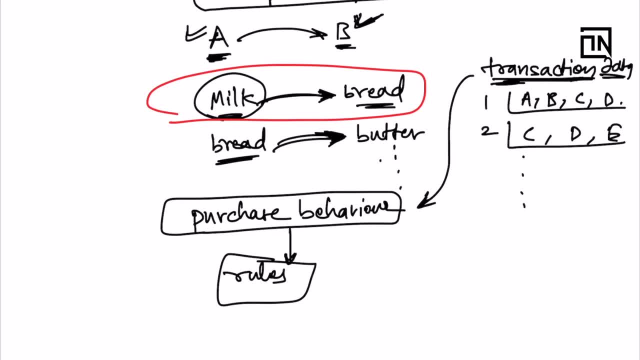 to help that. we have certain algorithms at place which can go through these transactional data and help us find out that. okay, these are some of the rules which are important, so please act on these rules. another very important, relatable example of this is like the changing of the shelves of products in the super stores. 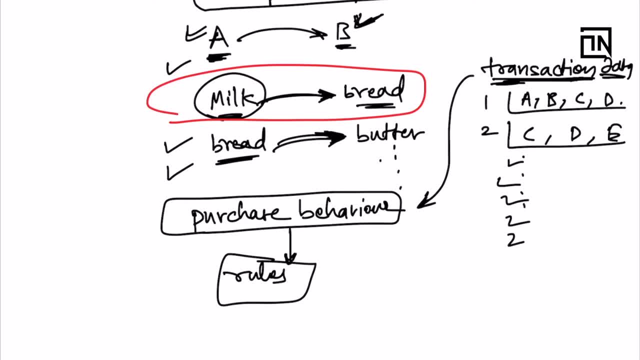 that is also based on two causes. there are two forces behind it. one is like the sales of prime locations at these super stores. companies pay these stores to keep their product highlighted: the ladder rack or the gondola and or the center table. they all have a particular price tag. 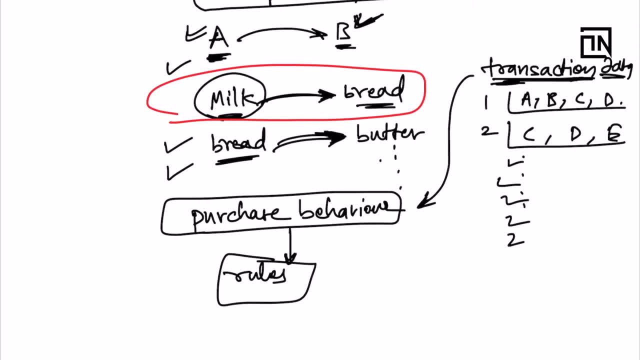 associated with it. so so manufacturing companies like cpg or nestle or procter and gamble, they will pay to these companies like dmart or walmart or tesco, to highlight their products. so that is one part of the story, but apart from that they themselves will do certain kind of association. 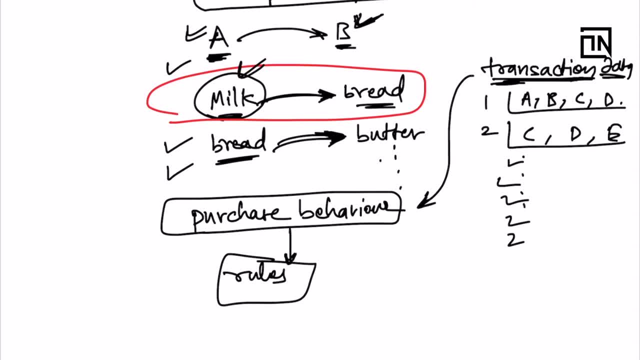 rule mining and they'll try to understand that, okay, milk should be placed near to bread, or or bread should be placed near to butter. so if i place these two item together in the shelves, the customer might see them and they and then they'll realize, oh, i have to buy this as well. 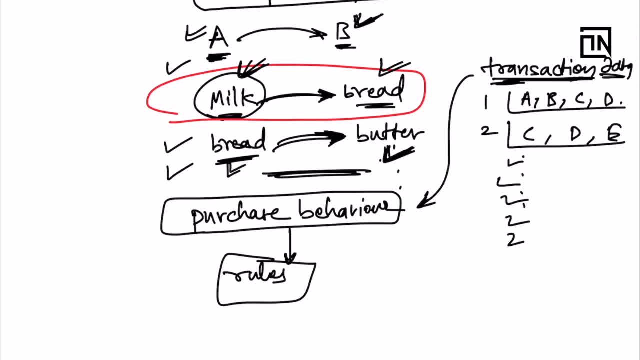 so their buying decision will be influenced. so this, this influence, is what we are trying to change. this, this buying behavior, is what we are trying to change by analyzing the purchase behavior of all the other customers. okay, we are trying to just just give a nudge so that the customer buys more. 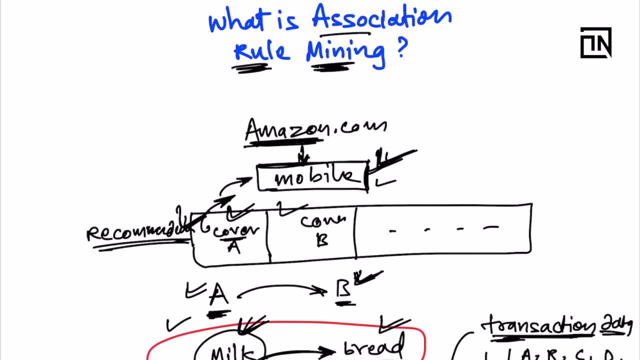 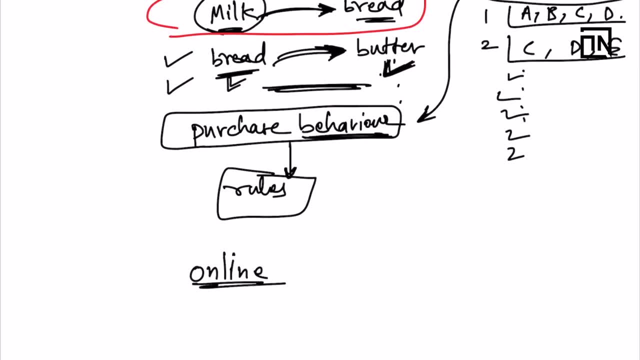 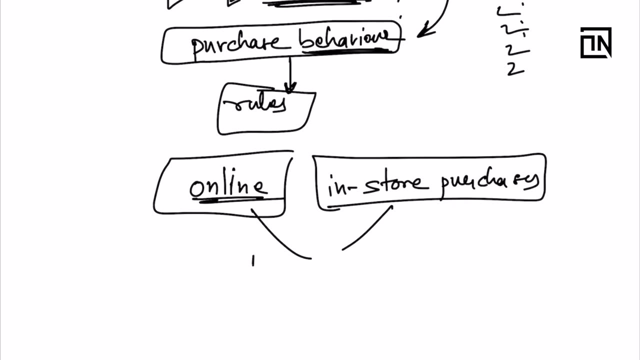 okay, now when do we utilize association rule mining? so, as the example says, whenever you have transactional data, it could be an online platform or it could be in-store data. wherever you are, you have these transactions data and using these transactions data, you generate rules. so you 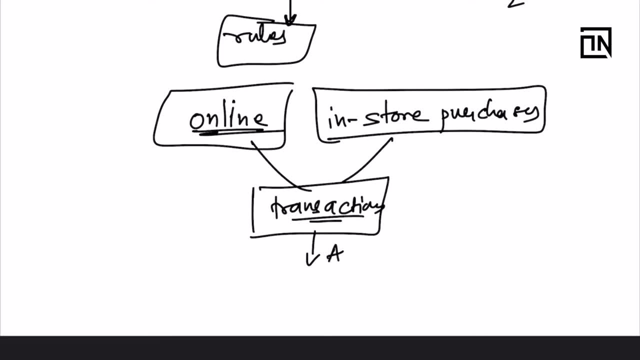 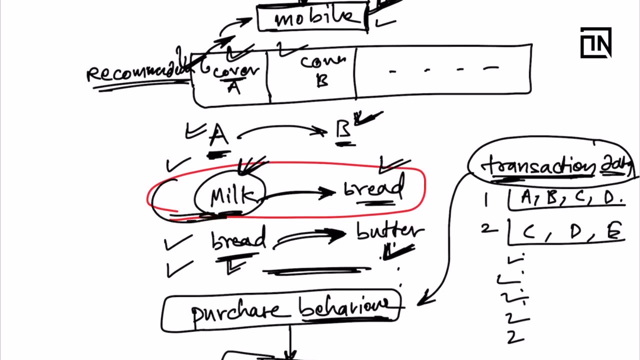 pass these two association rule mining algorithms, it will generate rules for you what you will do with these rules. so, once you understood that these are the rules present in my data, so you'll start acting accordingly, like if you know that your milk and bread should be placed near to bread or 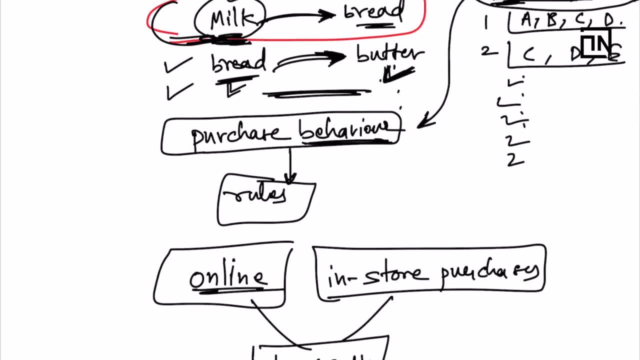 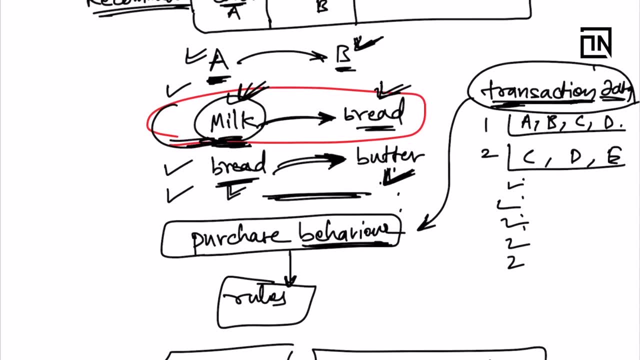 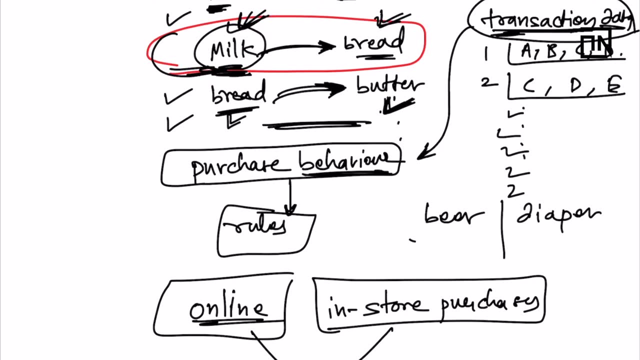 or let's say, let's say, a rare combination like milk and saffron should be placed together, or or curd and bread should be placed together, because people are buying. there is a very famous example called beer and diaper should be placed together, something like that. so 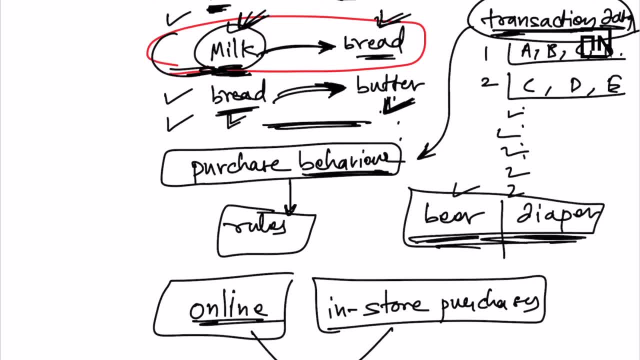 so you can't really imagine. but if people are purchasing this together, then definitely it makes sense to keep them nearby so that people purchase them okay. so sometimes some of the rules may not make sense to us, but if people are somehow purchasing certain kinds of products together, then we must try to act on it. we must try to use that information to 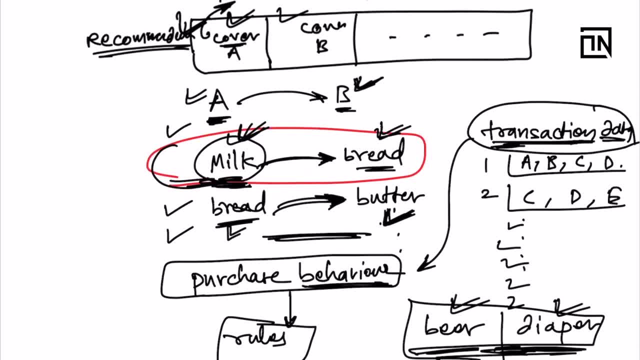 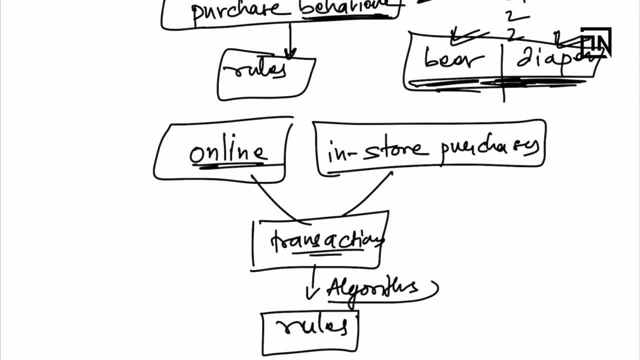 affect the buying decisions of new customers. if we make these rules just by our common sense, we will miss out on a lot of rules, and this is exactly where these algorithms comes into picture, because they can look through a large amount of transactional data and sort them and give you back the final rules which you should act upon. all right, so what are these? 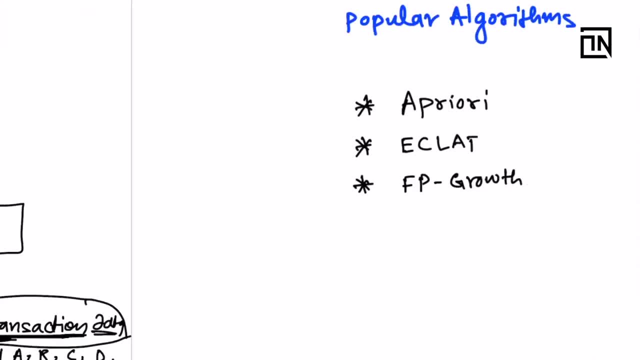 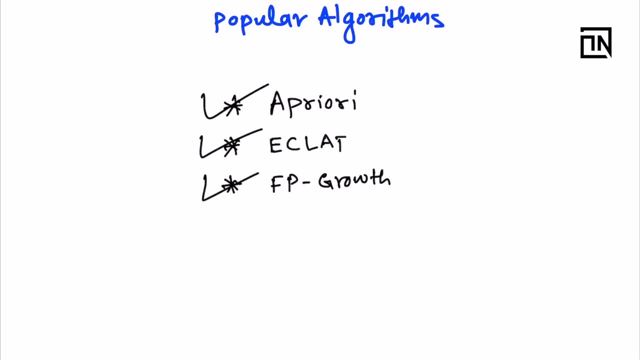 algorithms which can do association rule mining. for me so the popular algorithms in machine learning are apriori eclat and fp growth. so all these three algorithms are really popular for association rule mining. and all these, all these three algorithms have a basic set of calculations running behind. 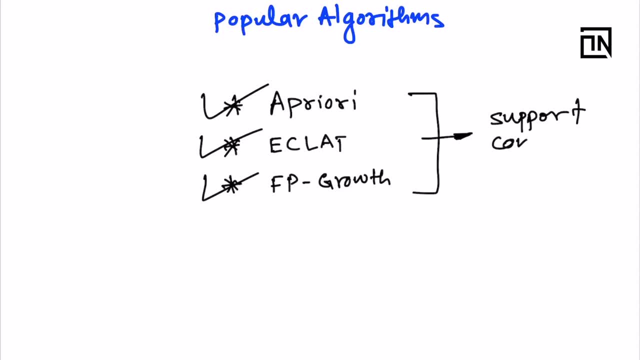 which is the calculation for support, calculation for confidence and lift. so these three things are calculated at the back end, for apriori also, for eclat also and for fp growth also. so if you, and if you understand what is support, what is confidence and what is lift, you have understood. 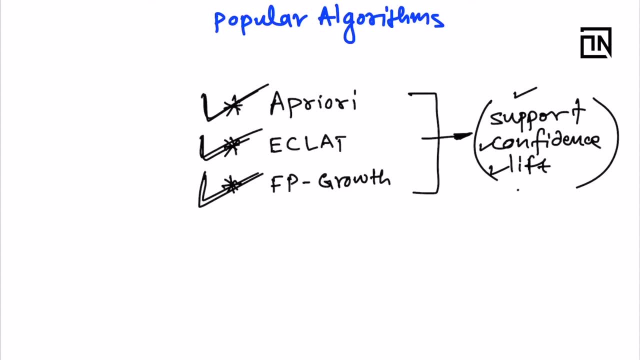 half of these algorithms. now, on top of this, there is a custom logic which runs in apriori, which generate rules. eclat also runs its own of improvised set of steps which will generate rules, and FV growth also is an improvisation. so so they work slightly differently from each other, but at the back end, the first thing they 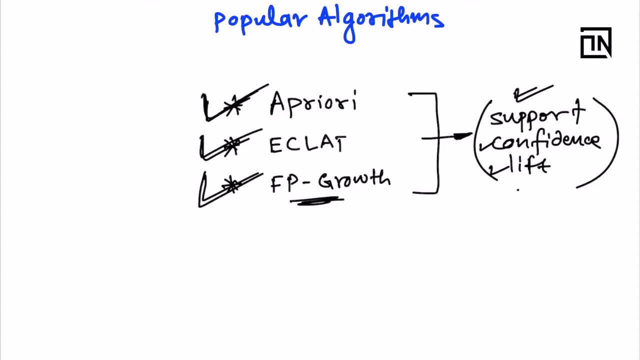 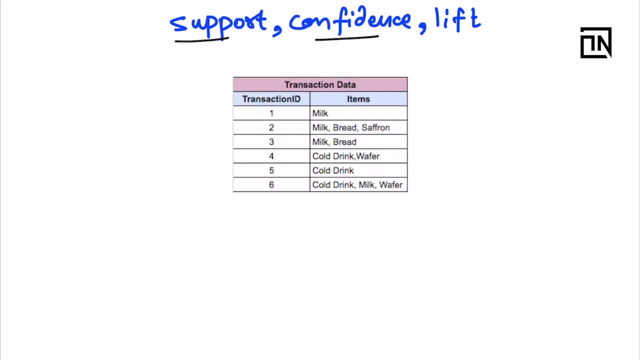 calculate is support, confidence and lift. so now let's try to understand these three metrics which are very, very important from association rule mining perspective. so support, confidence and lift can be understood easily by looking at a sample transaction data like this. so here, what I'm saying is transaction number one has happened where a person purchased only milk transaction. 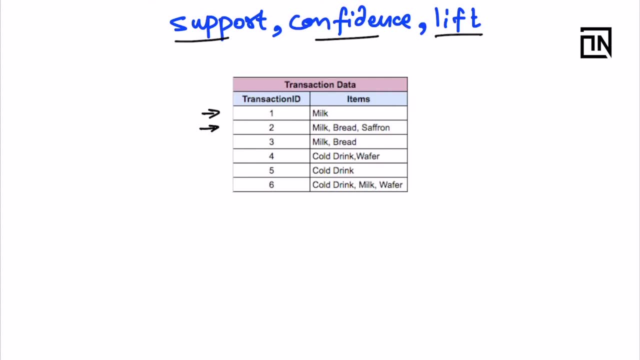 number two has happened, where a customer came and they purchased milk with bread with saffron. transaction number three: only milk and bread was purchased, so on and so forth. so there could be thousands and thousands of such kind of transactions. some people are buying a lot of stuff. 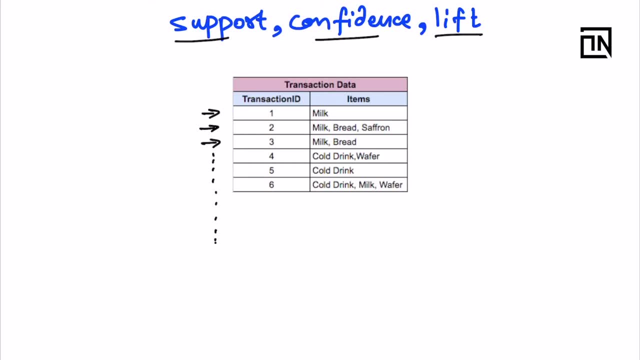 some people are buying only only one or two products and then they are going away. so, considering all the transactions, okay, in in this example, let us consider only these six transactions, so that our calculations are easy to understand and the same calculations are applicable everywhere, like once you have. 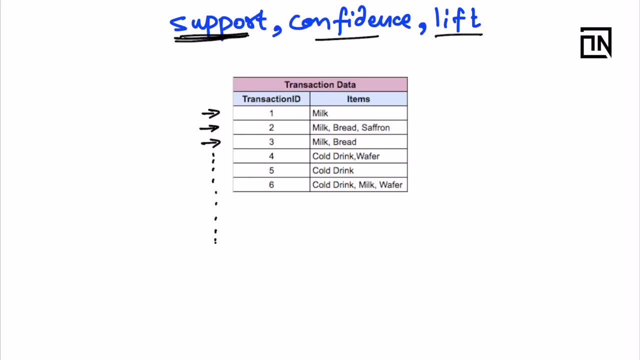 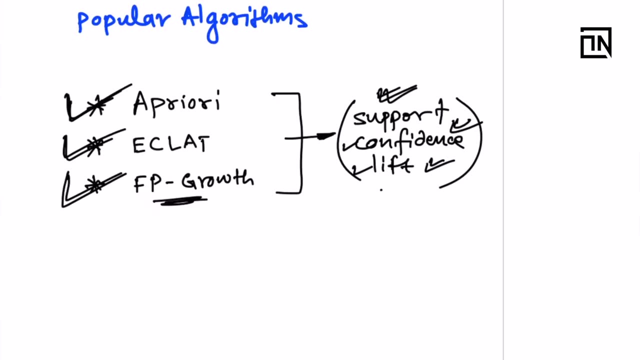 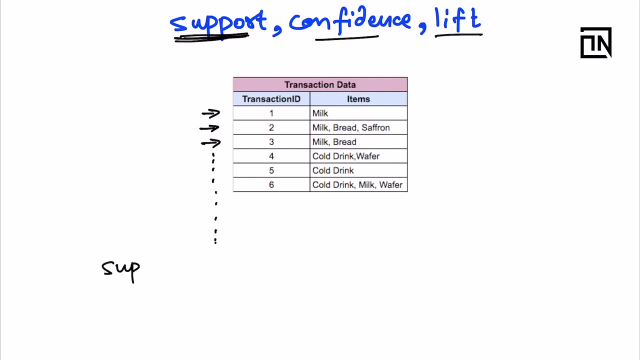 once you know how do you calculate support, that is applicable for any number of transactions which you have, and these are all very, very simple calculations based on counting. so all of these things are based on simple counting. so so let's, let's try to define support. let's say support. 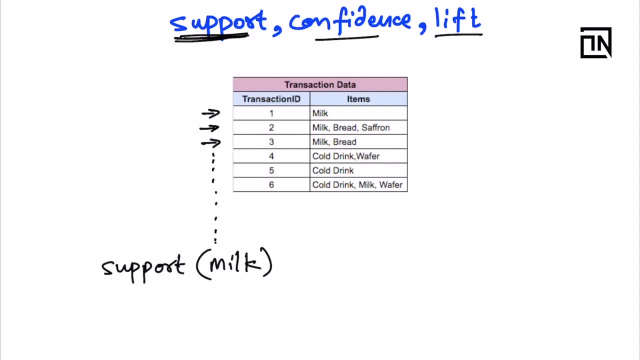 and of milk. what is the support of milk in these six transactions? so I'll just count how many number of times milk was present in these transactions. so transaction number one, transaction number two, transaction number three and transaction number six, these are the four transactions where milk was present divided by how many total transactions were there six. so four by six is the support for. 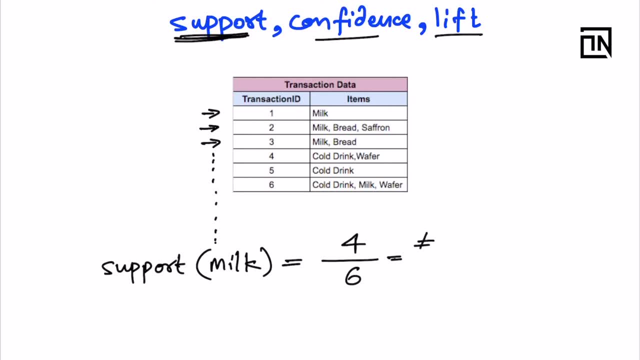 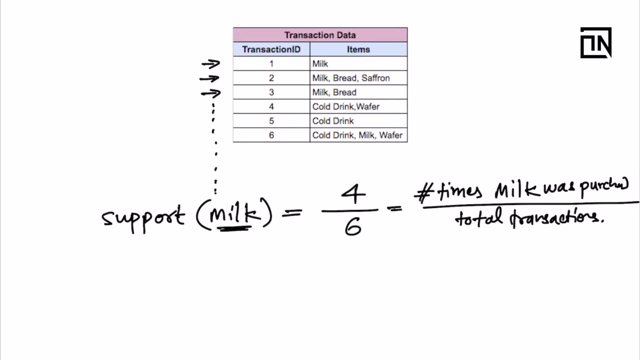 milk can be rewritten as number of times milk was purchased, divided by total transactions. similarly, it is not only for one product. it can be calculated for multiple products, like support of milk with bread. how many number of times do you see milk and bread together in these transactions? so transaction number two, transaction. 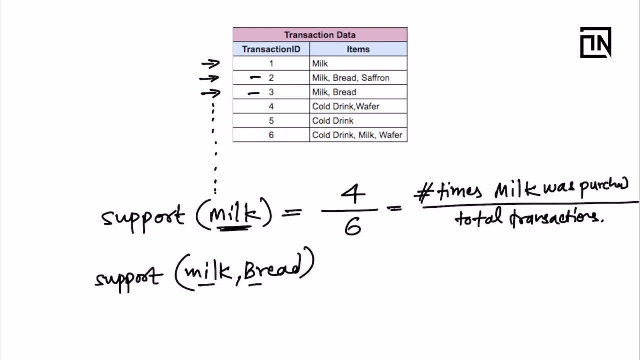 number three. that's it. so in two places milk and bread are present together, so I'll say two times out of all the transactions, so two by six. similarly, you can calculate the support of three products together as well, like cold drink- uh, cold drink, milk and wafer. what is the support for this? 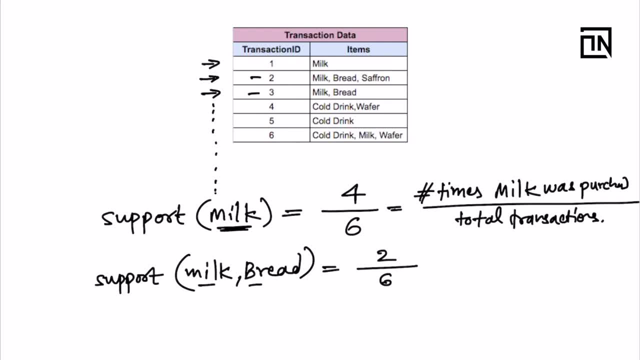 combination. it is one by six because it is being purchased only once in these six transactions. okay, so support really gives you an idea about how frequent these products are being purchased out of all the out of all the transactions. so four out of six times, or two out of six times milk and bread. 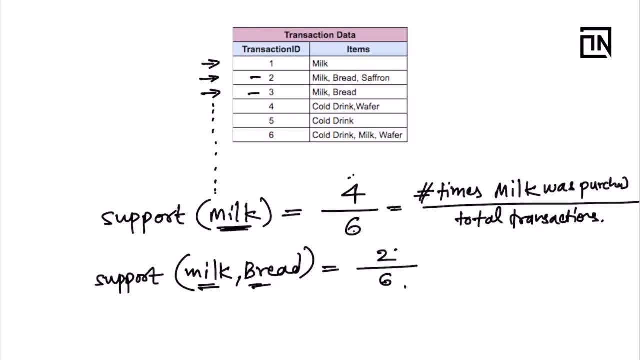 together was purchased, or four out of six times milk was purchased, or one out of six times cold drink milk and wafer together was purchased. so this gives you the support or the frequency with which you are buying one product or a combination of products. now the next metric is: 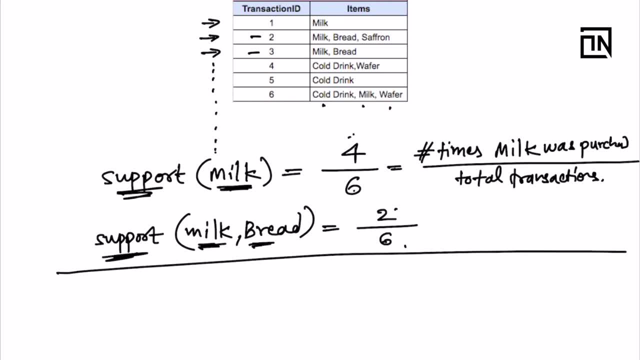 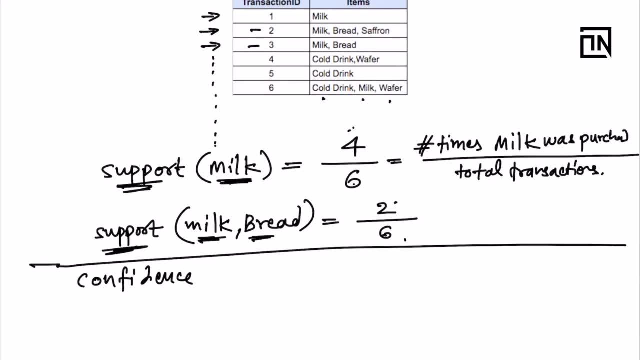 confidence. so confidence says, let's say, the confidence of a person buying bread if they have purchased milk. let's say milk leading towards bread. so when we calculate confidence we talk in terms of rules like this is a particular rule like person who is purchasing milk will also purchase. 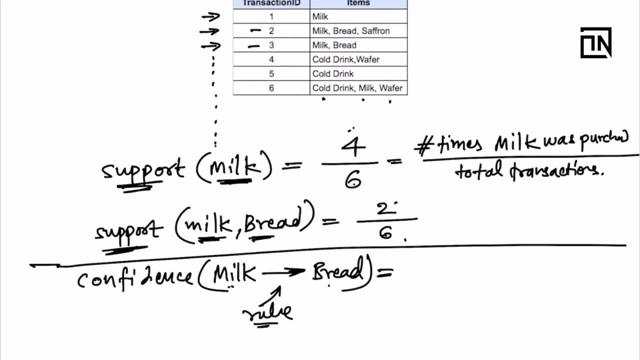 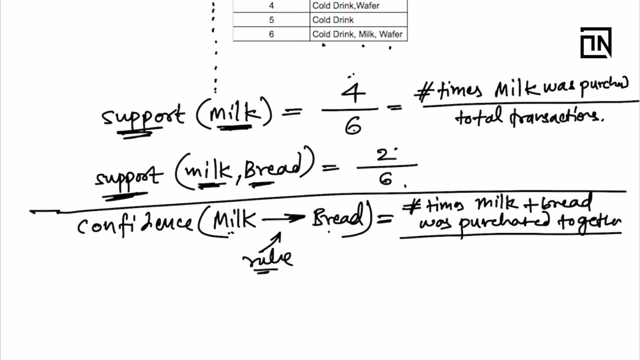 bread. so how do we define this? the number of times milk and bread were purchased together. number of times milk plus bread together, divided by now- this is important- the denominator changes when you calculate confidence. what is the denominator now? the denominator would be how many number of times milk was present. 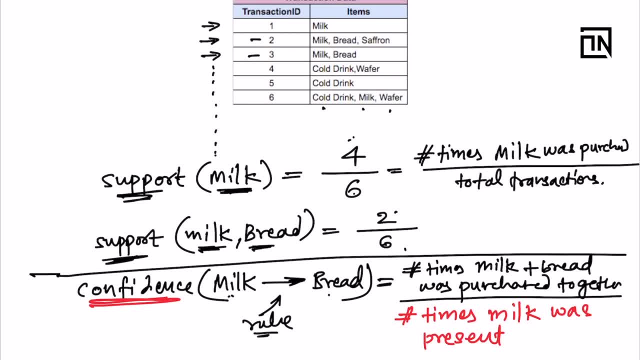 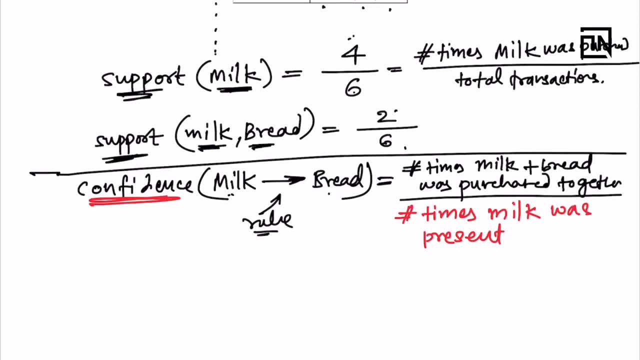 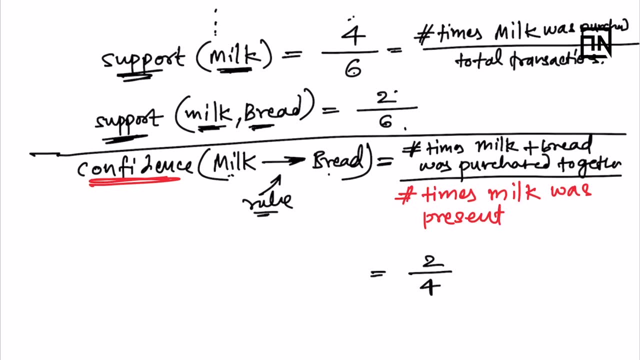 so in this data, how many number of times do we have milk? so transaction number one, transaction number two: three and transaction number six out of these, four times, how many number of times did milk and bread were present together? two times. so two by four would be the confidence that if a person purchases milk, that person will also 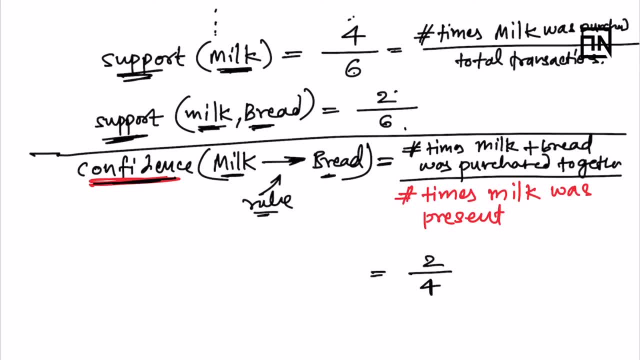 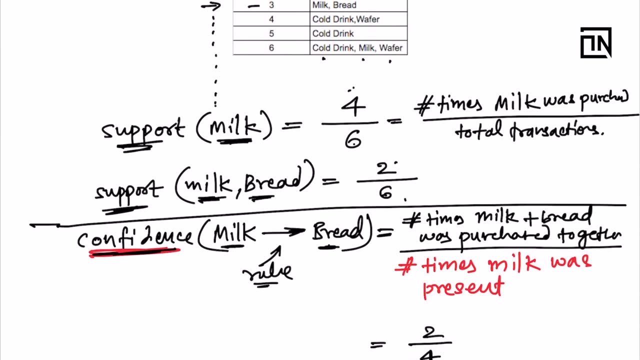 purchase bread. so two out of four means like just half. so there is a 50: 50 probability that a person who is purchasing milk will also purchase bread. okay, this talks about confidence. now this can be generated for different permutations and combinations, like, instead of having only one value in the left, 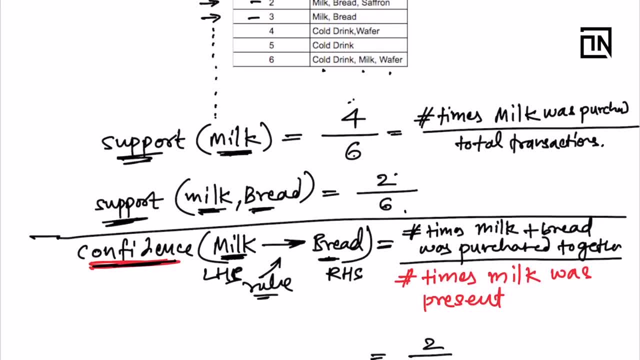 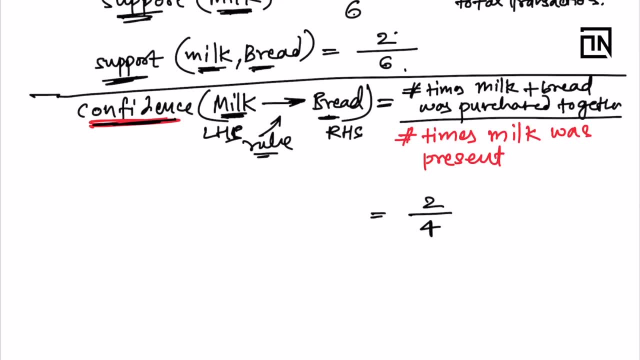 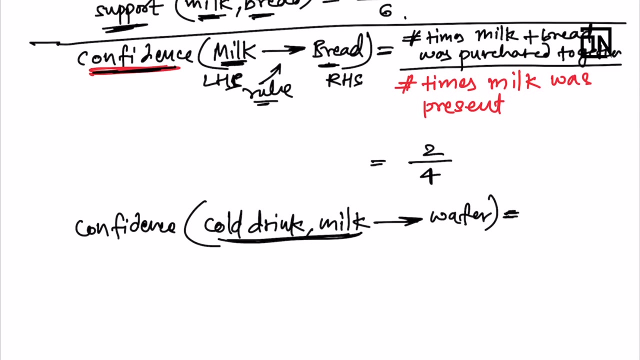 hand side and one value at the right hand side. you can have different values. let's say over here: what is the confidence of cold drink and milk leading to wafer? so confidence and milk leading to the two items are collectively leading to wafer. how I will calculate this? how many number of times? 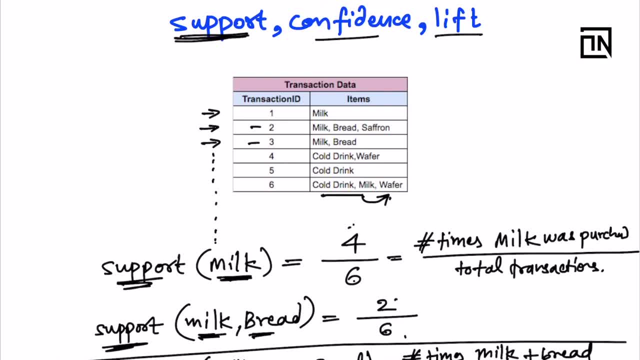 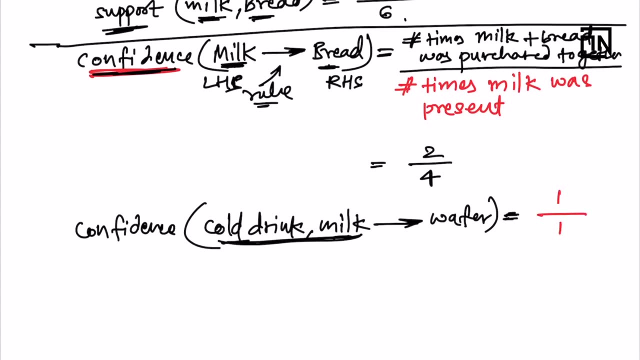 cold drink and milk were present together. so one cold drink and milk were present only one times. I guess, yeah, so here it is present only one times. so out of those one times you purchased wafer together, so one by one hundred percent now if I, if I have to shift, 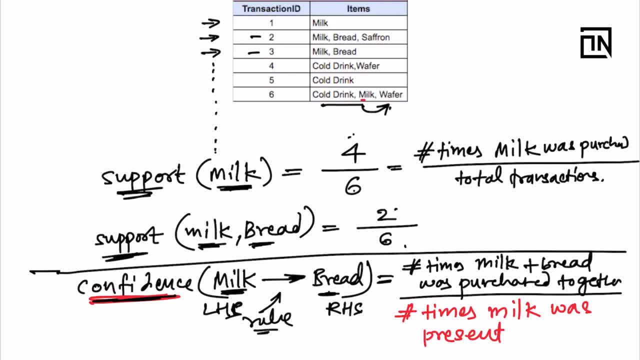 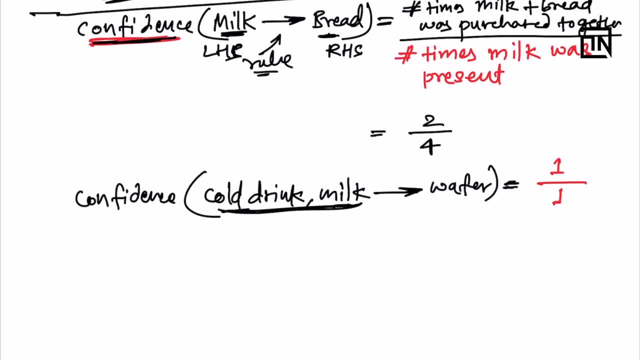 it a little bit to help you understand. let's say: uh, cold drink and wafer is leading to the purchase of milk. so the confidence equation will change. cold drink and milk- sorry, cold drink and wafer, these two items are leading to the purchase of milk. so if a person has purchased cold, 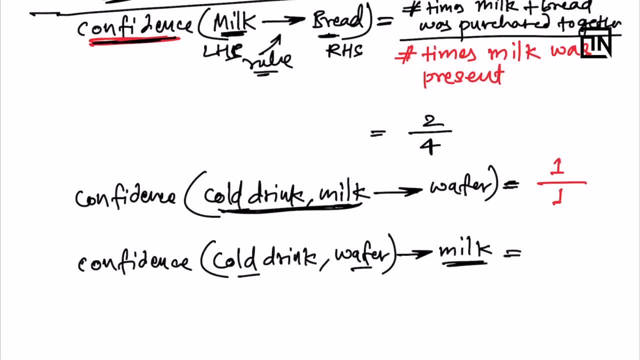 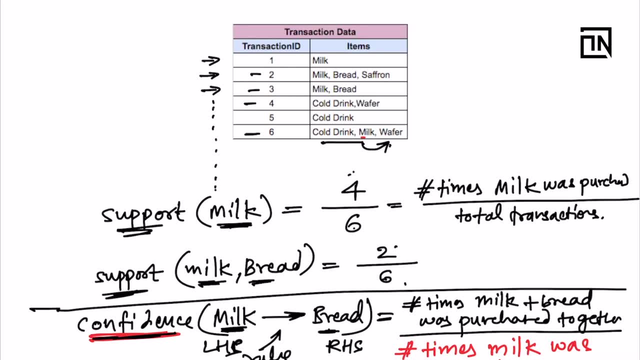 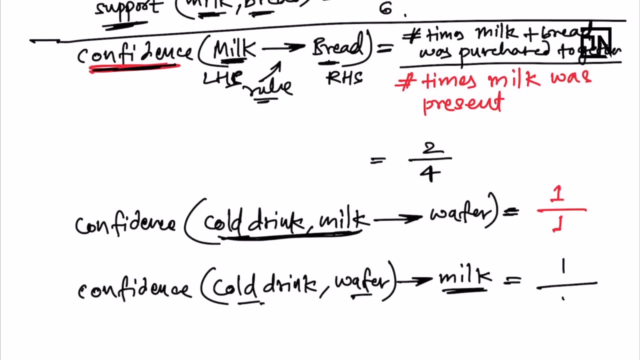 drink as well as wafer, how likely that person is to purchase milk. so how many number of times cold wafer were present in this transaction? so once in sixth transaction and once in fourth transaction- and out of these two transactions how many number of times milk was also purchased? one times, so 50. 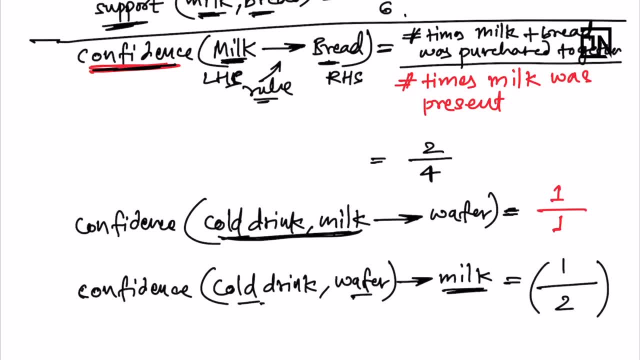 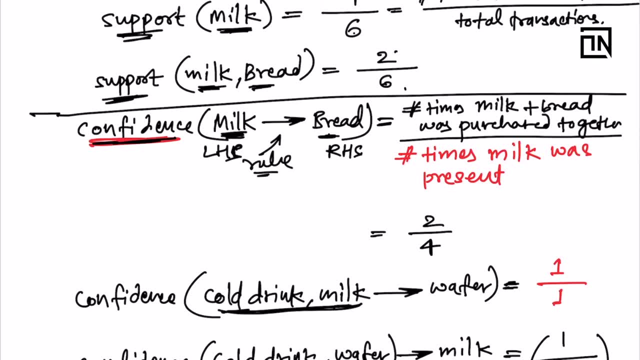 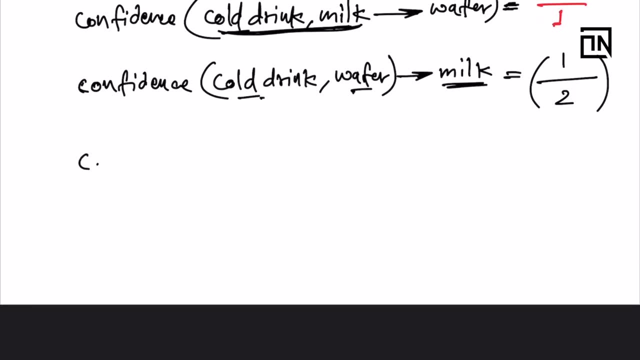 probability. now, the moment you reverse the confidence equation, then also the values change, like like this milk and bread example. so the confidence of milk and bread would be different from bread and milk, like what will be the confidence over here of a person who is purchased bread first to purchase milk. so now the equation changes. now i will have to understand it in terms 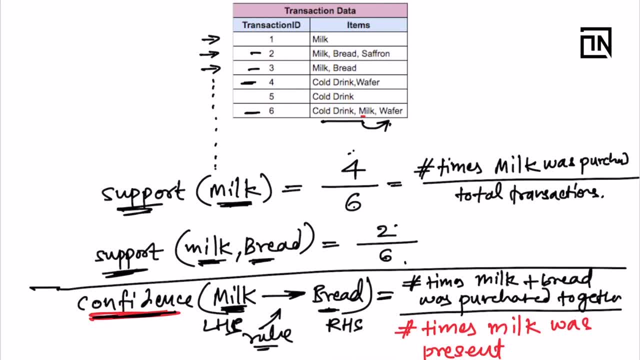 of how many number of times bread is present in my total transaction. so where, where, where is bread present over here? to two times, and out of these two times, how many number of times milk was also purchased two times, and out of these two times, how many number of times milk was also purchased. 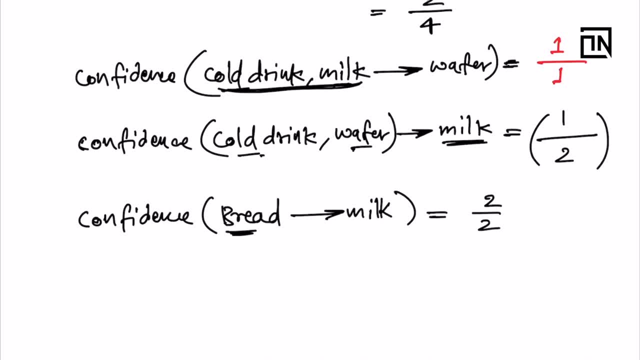 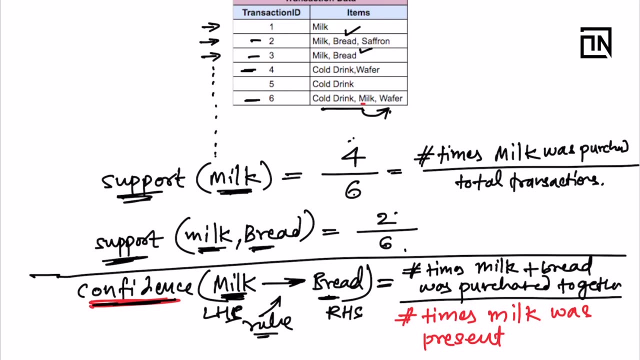 two times. and out of these two times, how many number of times milk was also purchased two times. so, hundred percent of the time, if a person has purchased bread, they are very likely to purchase milk, definitely because two out of two times you have purchased uh milk over here. okay, while while 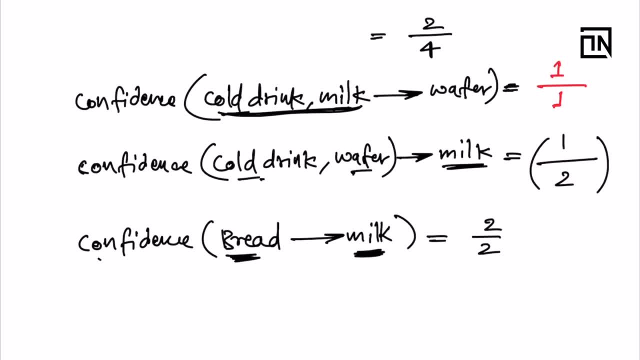 bread was purchased. so so this is how you calculate confidence. now, confidence talks about how confident you are that a rule will occur or a rule will happen. so these fractions are nothing but probability. you are calculating probabilities, that how probable is this event or is this rule to happen? so you count and then you calculate the probability. so confidence works. 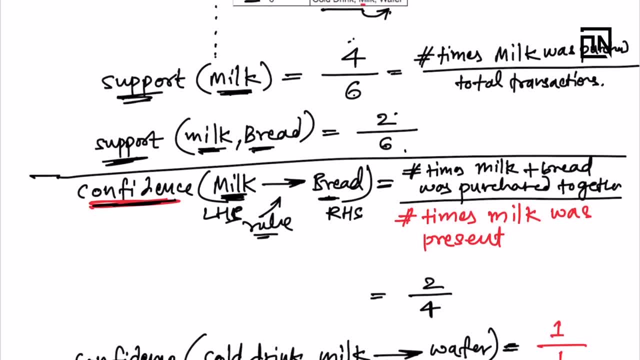 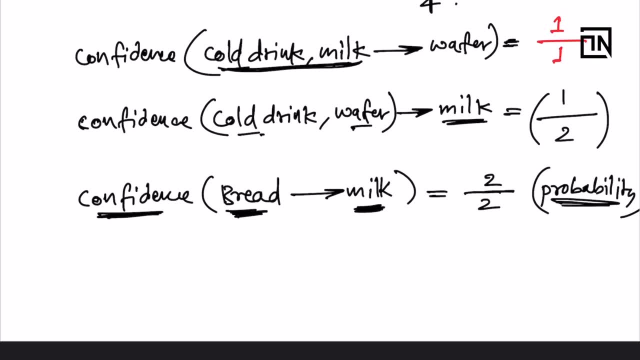 both ways. so if you have a confidence of milk leading to bread, that is different. it's two by four now and bread leading to milk. this is different now. now you have two by two or hundred percent probability. so confidence: if you change the direction, the confidence value will change. 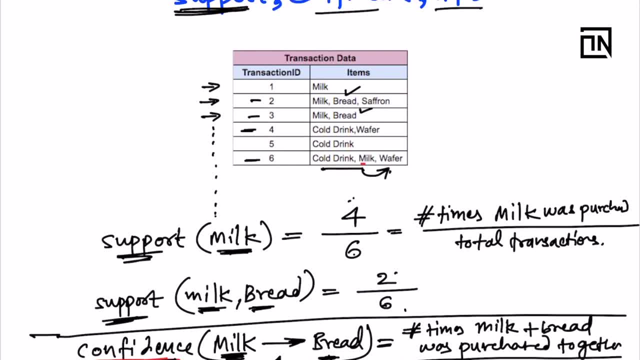 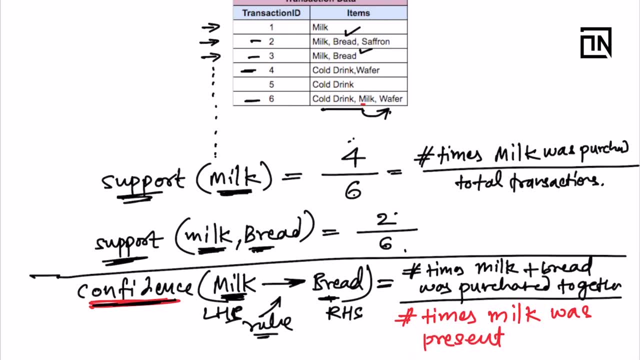 drastically. this is not the case with support. for support it is simple: counting from all the transactions. so that is why you say support of milk and bread purchased together or bread or milk being purchased together is same, it doesn't matter. you are just trying to see how many number of times 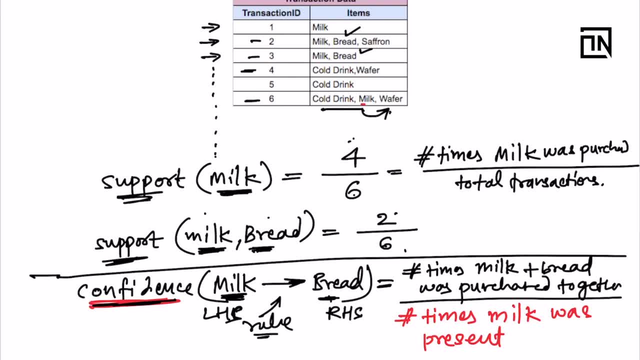 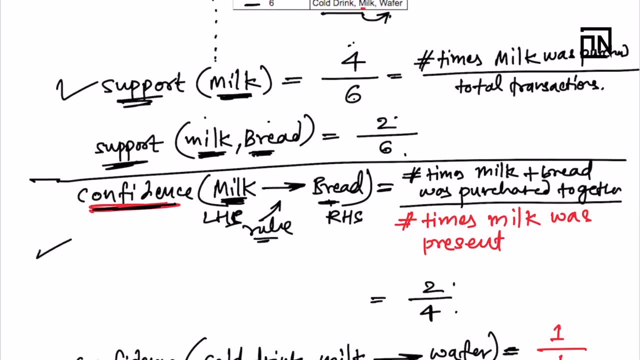 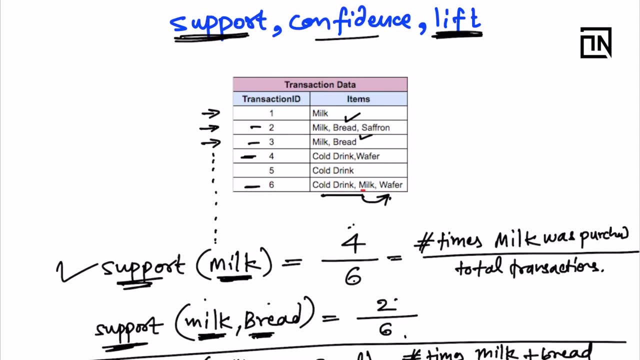 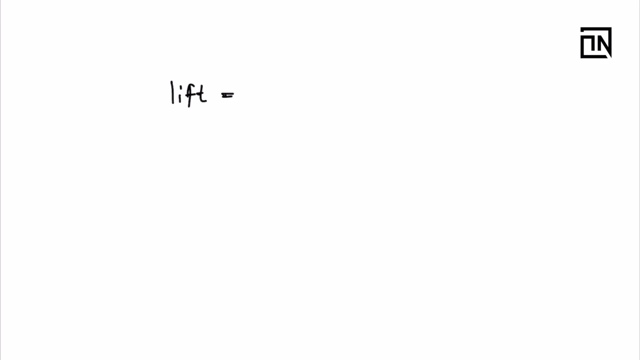 milk is present, along with bread divided by the total transaction. okay, so support and confidence, these two metrics are something which you can easily decipher or easily calculate, easily explain or understand. the third one, lift, is slightly tricky. what lift says is this: so lift can be defined as the lift of a particular rule, let's say, lift of a particular rule, a leading. 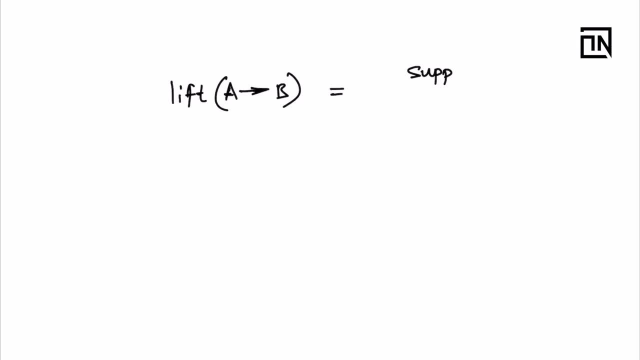 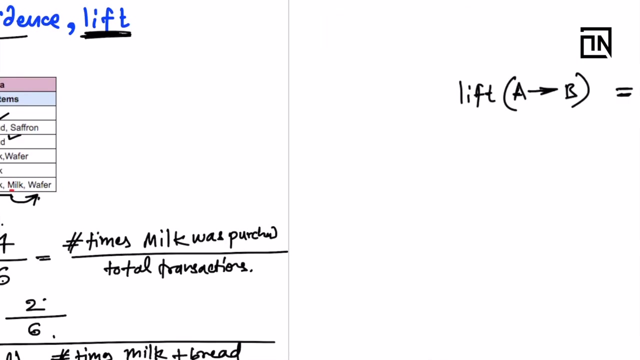 towards b can be defined as support of a and b being purchased together, divided by support of a and support of b. this is something which which cannot be easily interpreted, just like you have interpreted the support standalone and confidence, so this lift value can be interpreted based on. 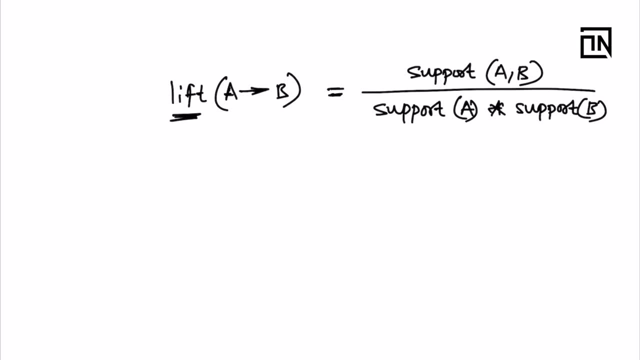 based on certain thumb rules, like if the lift value is greater than one, then it says if one pro, if one particular product has been purchased, the other product is also very likely to be purchased if it is less than one. if the lift value is lift value is less than one, it means if one product a or product a is. 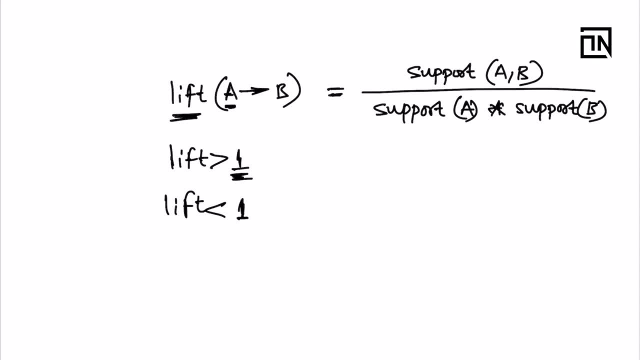 being purchased, then the other product is not likely to be purchased. we can say: a does not lead to b, or if a person purchases a, it means that they will not purchase b, or it is not very likely that they will purchase b. if lift is greater than one, it means a. 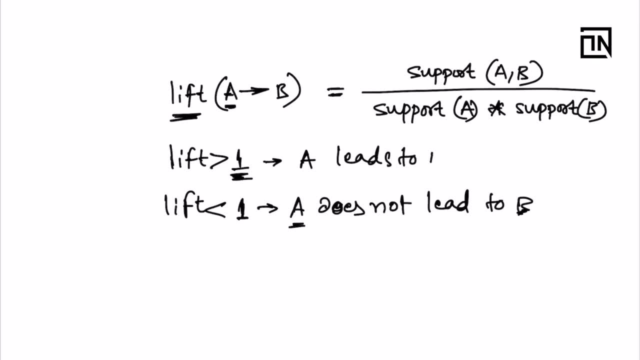 leads to b. so, using a, you you know when you are, when you are purchasing a, then you are very likely to purchase b. also, if lift is equal to one equal to one, then we say the products are not related to each other. a and b are not related. so there is no visible evidence that if a is purchased, then b. 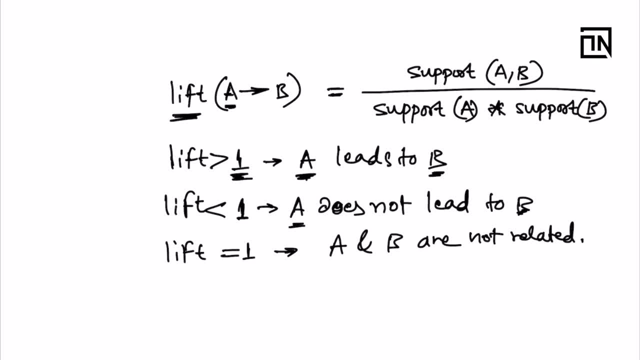 will also be purchased. or b- non-iv 1000 yen, non-iv 1000 yen- b is purchased, then a will also be purchased. so we say there is no association. okay, so these are the rules which you, these are the you can say values for lift which you need. 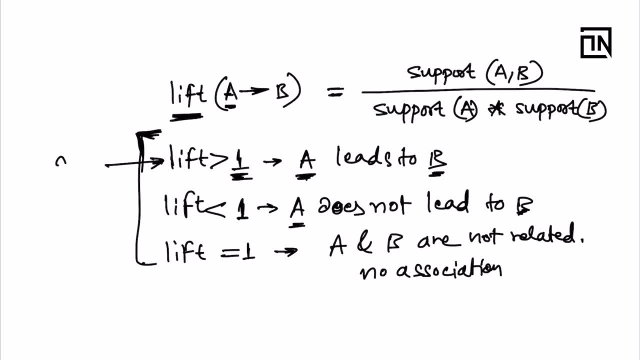 to keep in mind, and the good scenario is this: that the lift must be as high as possible from one, so that it represents that a is strongly leading towards b. so it's formulae support of both of them being together divided by support of a and support of b. now, if you do the calculation, 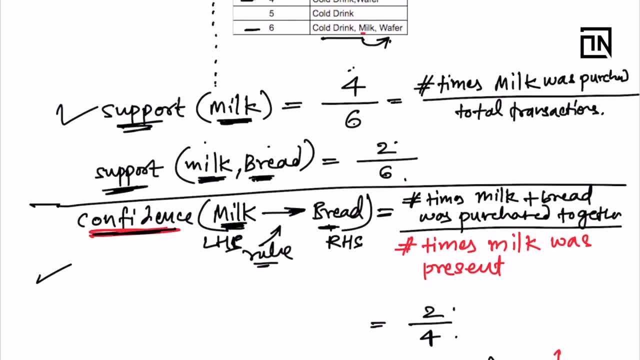 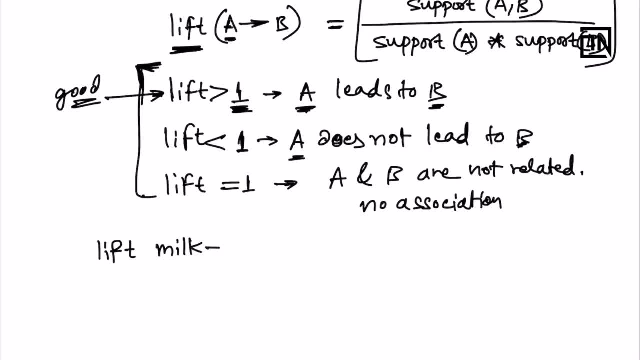 with with a previous example, like milk and bread example, so you can calculate the lift of milk leading to bread, as this support of milk and bread together divided by a and b- support of milk and support of bread, all right, so so using this formula, you will be able to calculate the lift. 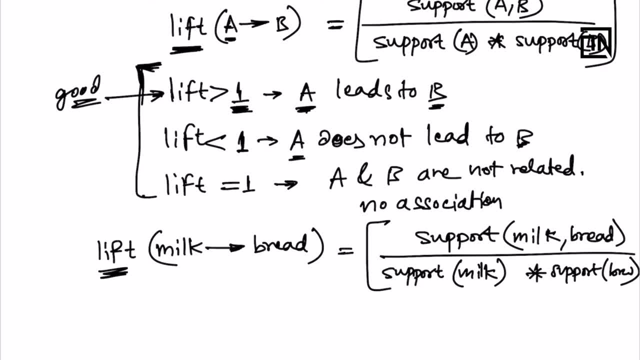 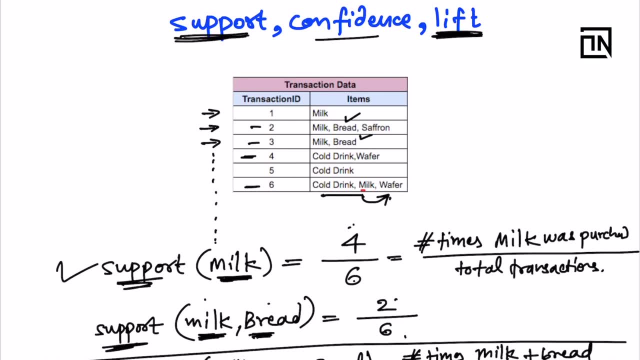 value of any given rule, any xyz rule. all right, now, when you take up a transactional data, you can kind of create so many different permutations and combinations of these rules, like milk leading to bread or milk plus bread, or milk leading to bread or milk plus bread, or milk leading to bread or milk. 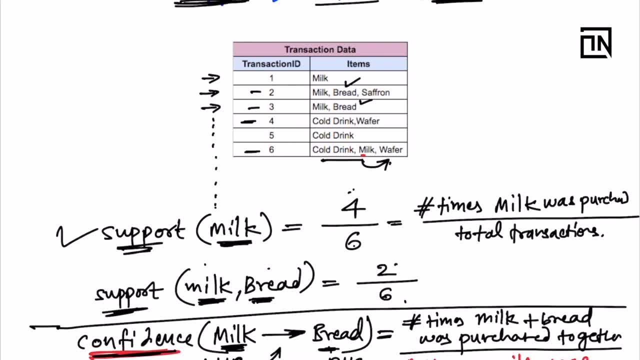 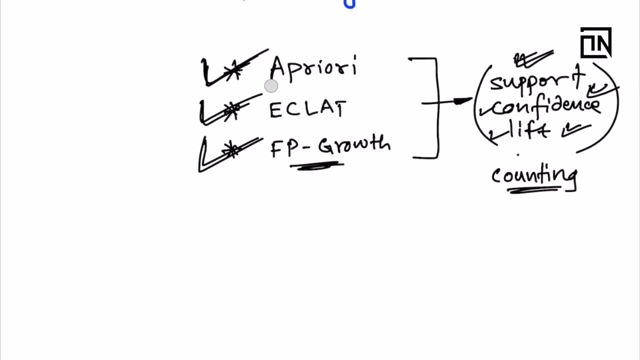 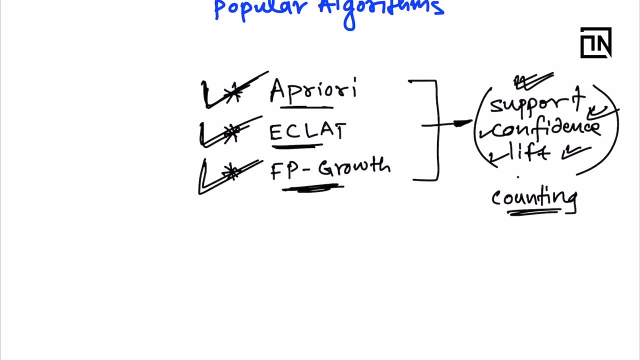 bread leading to saffron, or or bread leading to milk, or cold drink leading to wafer. so so there are endless combinations which you can create now, how apriori creates them, how eclat creates them, and how fp growth creates them. there is a subtle difference in between them, but at the back end, 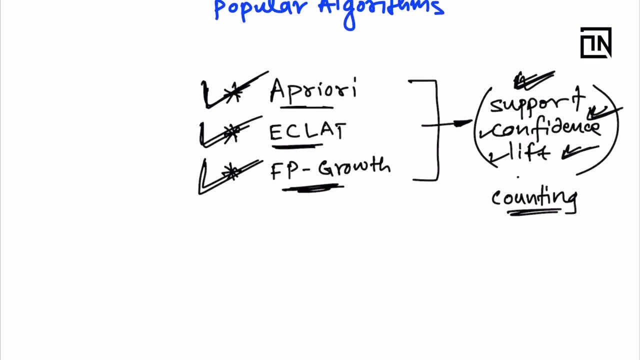 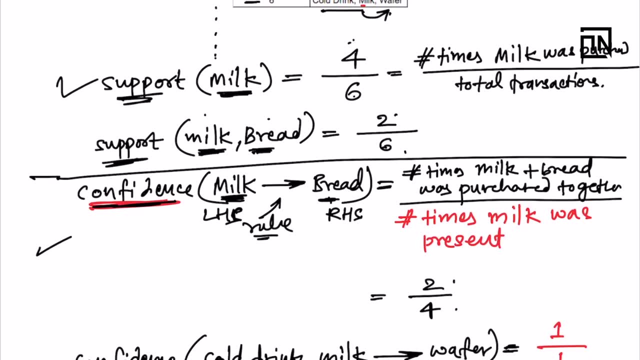 they will calculate support, confidence and lift of every prospected rule or every prospected association which they will try out. so there are a lot of combinations, but using certain parameters, using certain thresholds, we choose only those rules which are actionable. and how do we choose like? which particular rule is good for me? so typically the confidence should be very high. 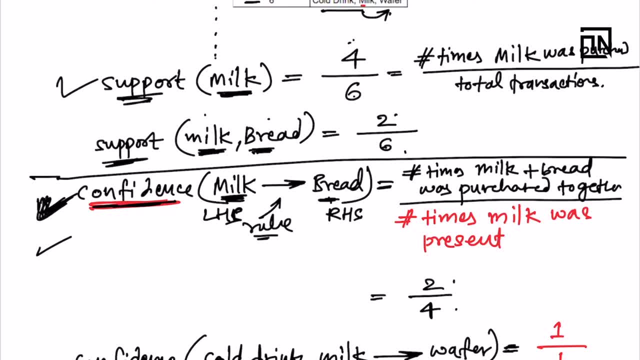 of that rule, the support could be low, but the confidence must be very, very high, like the milk and saffron example. so if, if somebody is purchasing um, um, sorry, uh, if, if somebody is trying to purchase saffron, so definitely they. they will have to. 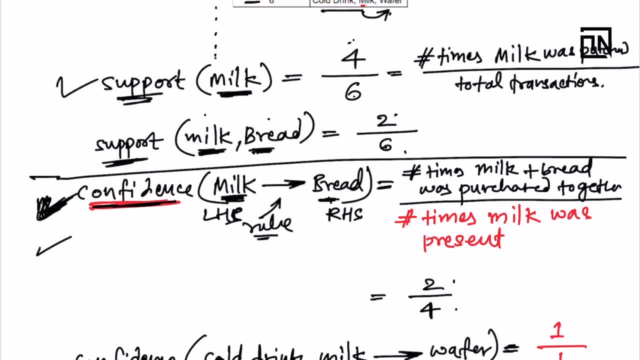 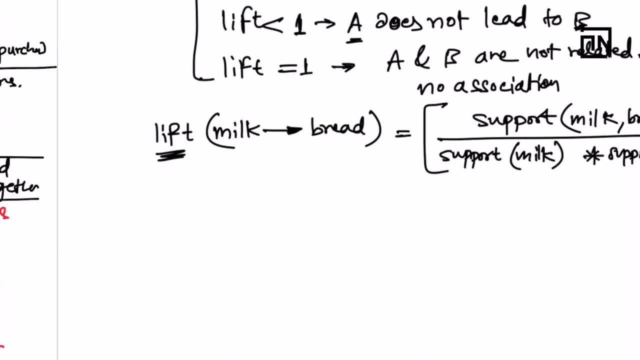 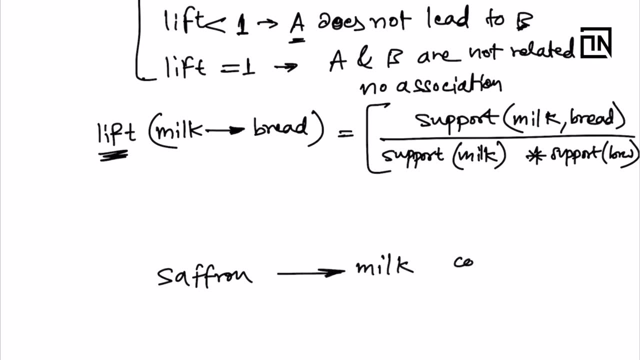 either drink it with milk or they are trying to make something on top of which they they would like to sprinkle saffron. so it's very highly likely that a person who has purchased saffron, the confidence of purchasing milk will be very high. so when a confidant, when a confidence of the rule, is very high, 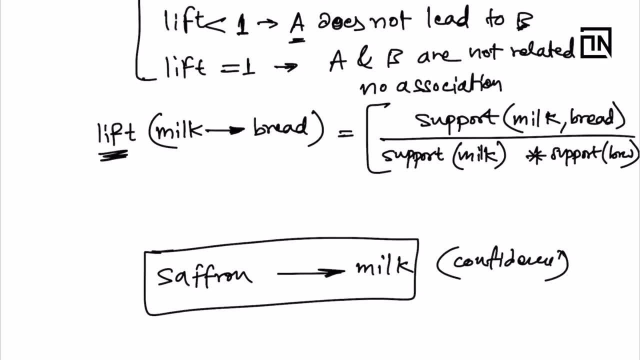 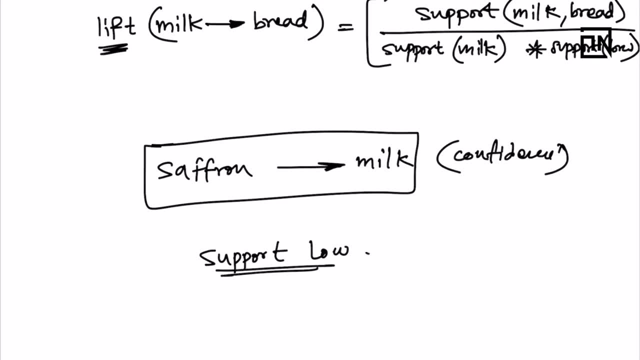 then it is actionable, even if the support is low. so low support means what? it just occurs rarely. and low confidence means what? that it doesn't occur in a way in which we are trying to protect, project it. one one product does not effectively leads to the other product if we just 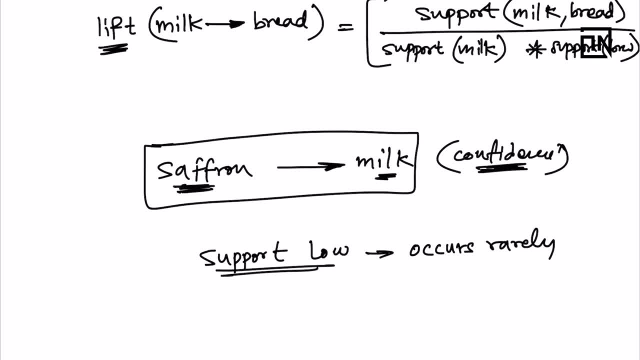 focus on only the purchases where saffron was included, then there are very less places where milk was also purchased. so so that will represent confidence. so confidence is something which tells you about, you can say, the strength of a rule. so i always need high, confident rules.